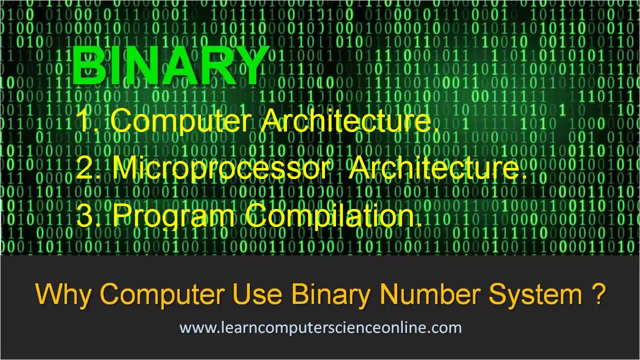 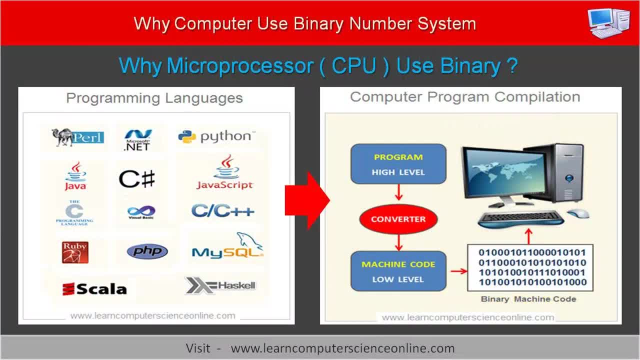 Let us now discuss each of these topic in detail to understand why computer use binary number system. at the hardware level, The computer system is an electronic device that can be programmed to perform various user specified operations. However, the computer system needs to be directed by using a set of instructions called program instructions in binary code. 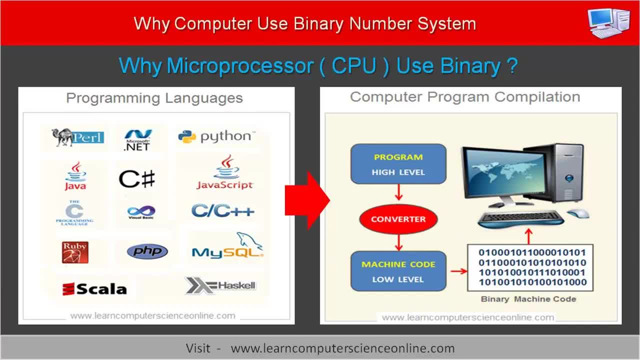 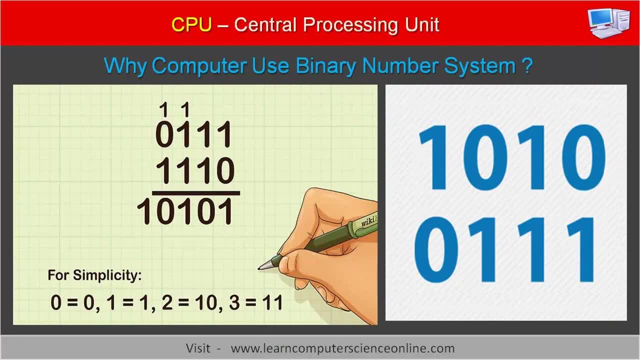 Let us now discuss what is binary number system. In mathematics, a binary number is used to represent any number using only two numerical numbers. that is equal to zero, And therefore the binary number system is said be a base two number system. 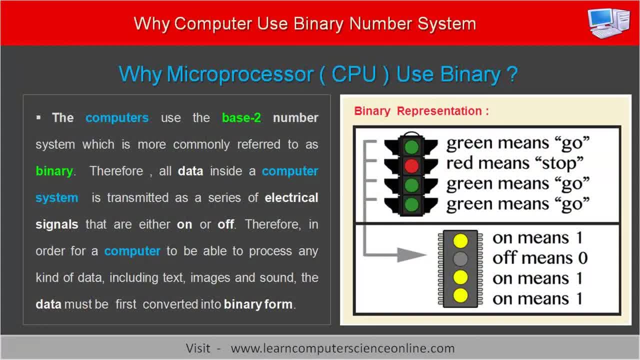 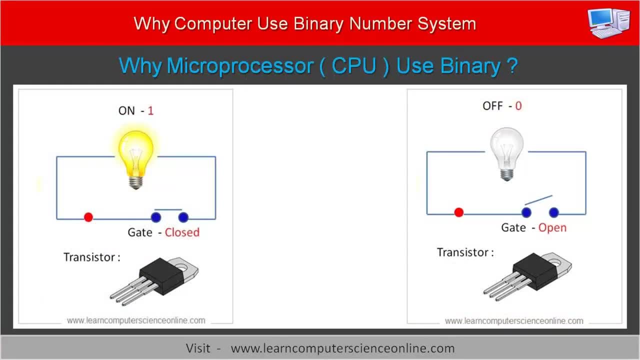 The binary number system is extensively used in the field of digital electronics, Mainly due to the ease of its straight forward implementation. The computer system is also a digital electronic device which consists of number of electronic components. In digital electronics it becomes very easy to define the two states, that is, on state and off state. 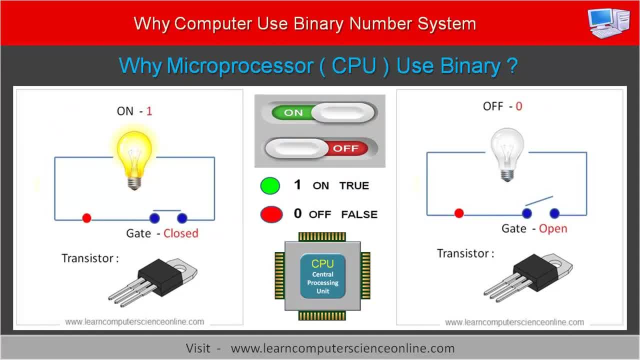 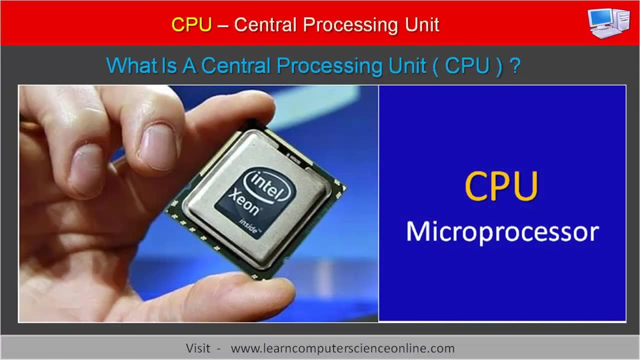 Using the binary equivalent. In order to understand the reasons why computer use only binary code, we need to first understand the computer system architecture And also the micro architecture of the central processing unit. It is the microprocessor that provides the processing power to the computer system and executes the program to perform any task. 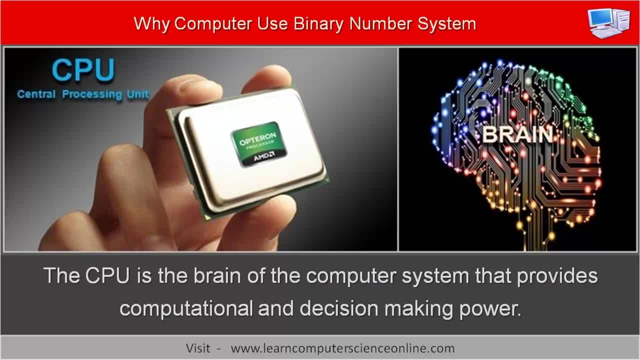 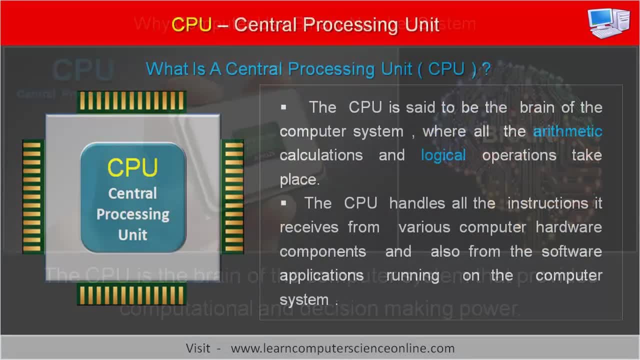 The microprocessor is the brain of the computer system, Which controls all the components, CPU operations and the program execution. The software consists of set of program instructions executed by the microprocessor, Which directs the CPU to perform the desired operations. 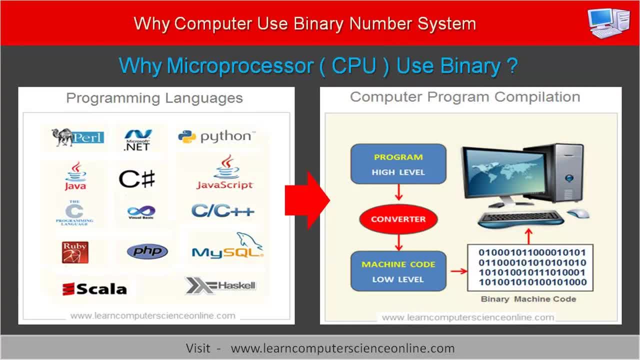 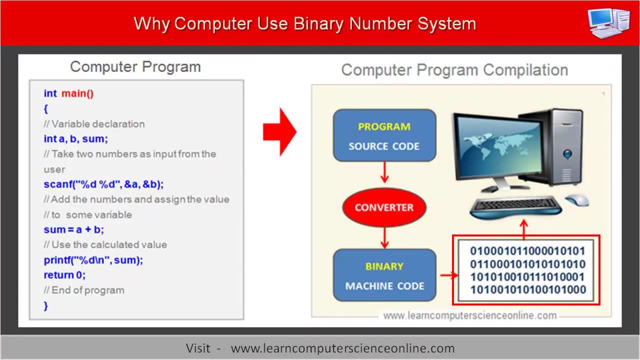 The computer programs are written by using a human friendly high level programming language Such as C language, C++, Java, Python And there are many such languages. However, since the microprocessor executes only binary commands, The high level computer program also needs to be first converted to machine code. instructions in binary. 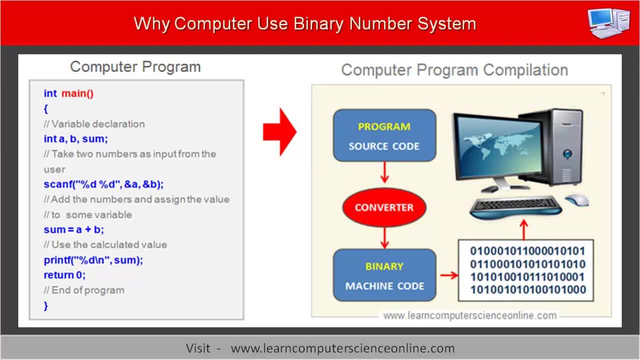 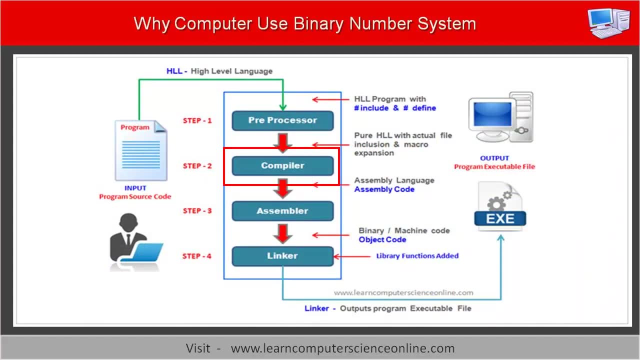 So it doesn't really matter which high level programming language you choose to write the program code, Because eventually all high level programs are required to be converted to binary code. This conversion is done by using a special program Called compiler. 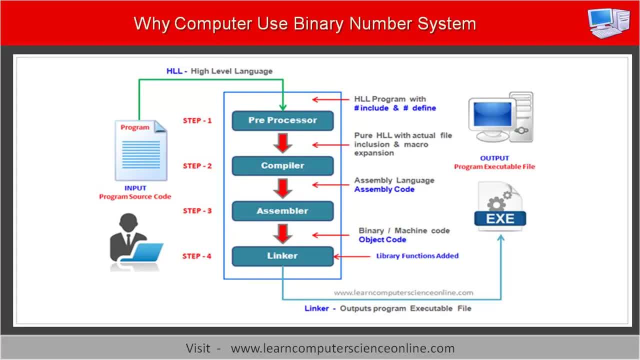 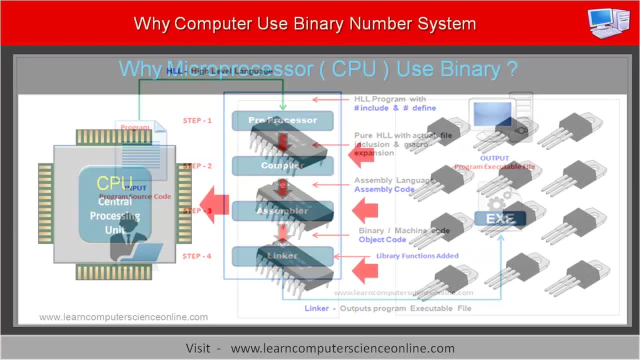 This conversion process is called the program compilation. During the program compilation the high level programs are converted by the compiler Into machine code instructions in binary That can be directly executed by the computer processor. The microprocessor chip internally consist of millions of integrated circuits. 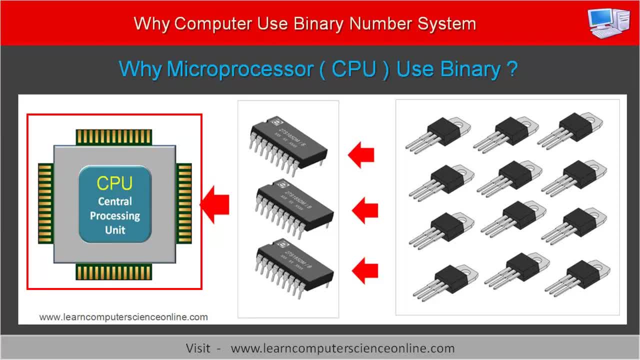 Packed in a microprocessor chip. This technology is referred as variable, A very large scale integration used in the processor chip. Each integrated circuit inside the processor chip consists of millions of tiny components called the transistors. 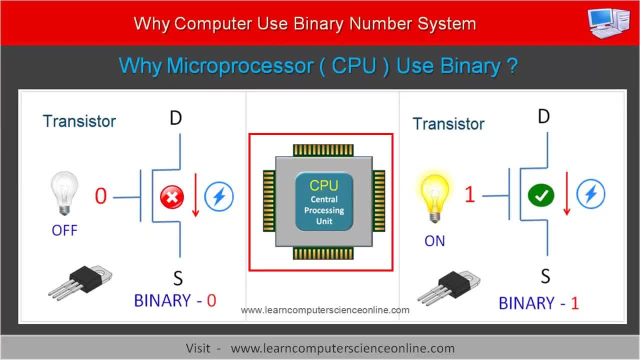 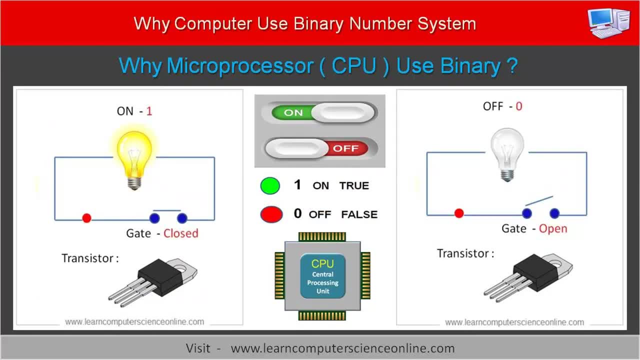 The transistor is a fundamental building block for all microprocessor chips. The transistors are used as microswitch inside the processor chip And therefore the microprocessor understands only binary language of 0, and 1.. 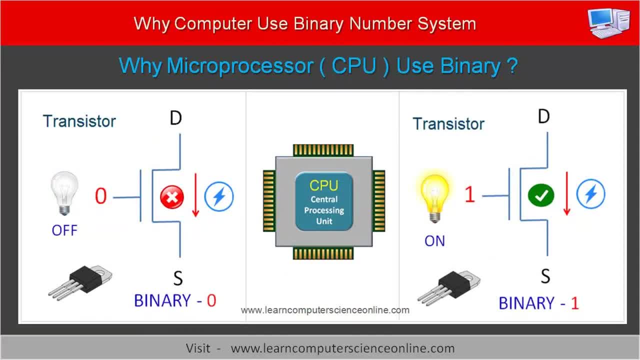 The transistor is made up of silicon, which is a semiconductor material. The transistors inside the CPU function as a microswitch That can be programmed to be in a either switched on or switched off state. When the transistor is in on state, it represents the binary number 1.. 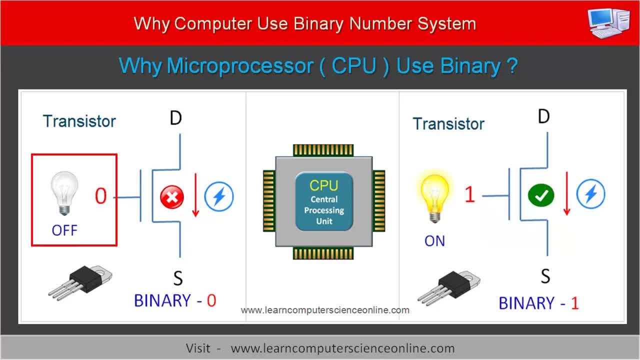 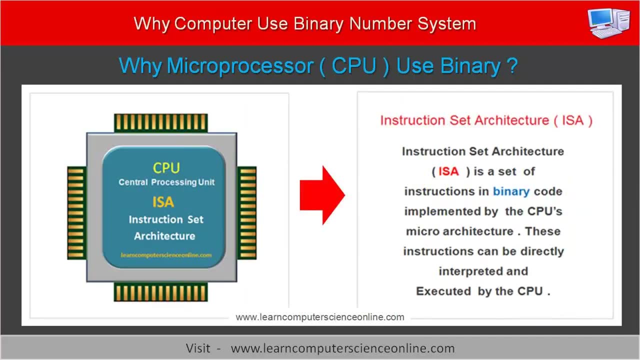 And when the transistor is in off state it represents the binary number 0. And for this reason the microprocessor within a computer system can be programmed to execute only program instructions in binary, Another important factor that makes the binary suitable for computer system. 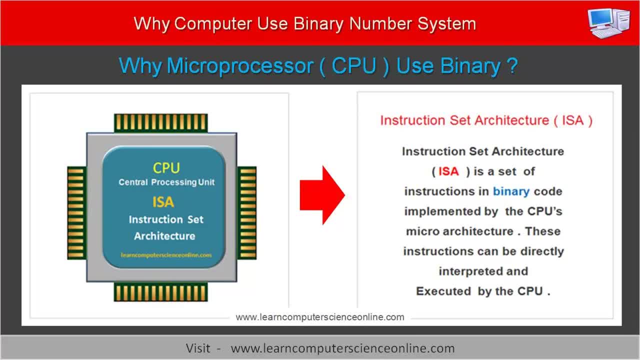 is the microarchitecture of the processor chip itself. Each microprocessor chip implements a microarchitecture called instruction set architecture. The instruction set architecture defines the set of commands in binary which processor chip supports The processor manufacturing companies design the processor chip.